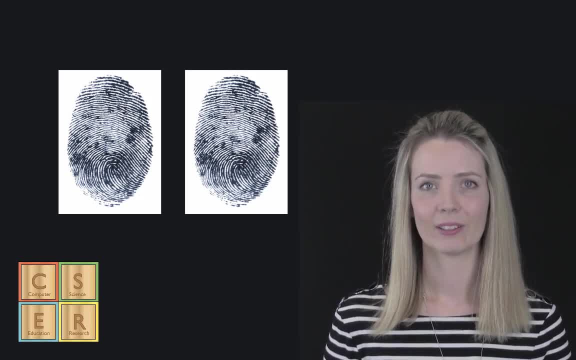 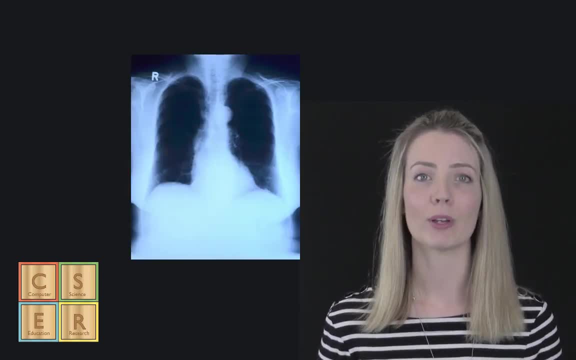 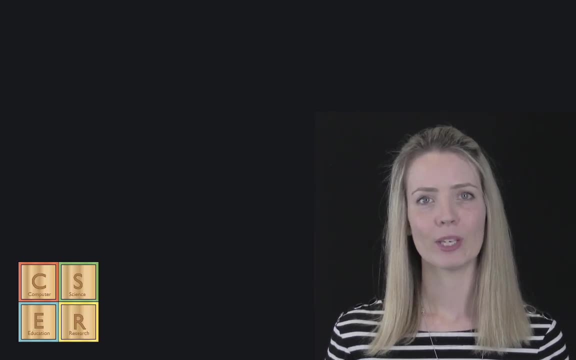 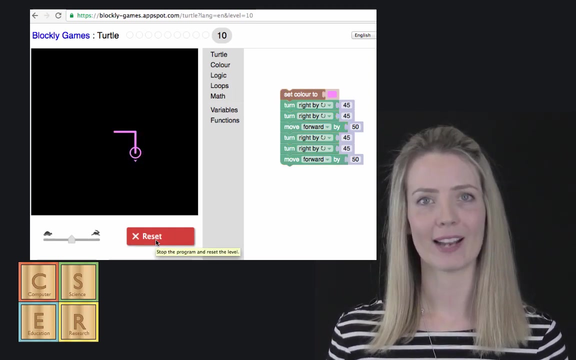 for example in fingerprint or photo identification, or in the medical sciences, by mapping similarities and differences in medical imaging, or even within commerce, by finding patterns in behaviour within big data. When using visual programming languages, we can use pattern recognition to identify the commonalities or repetition in our code, Instead of writing the same thing over and. 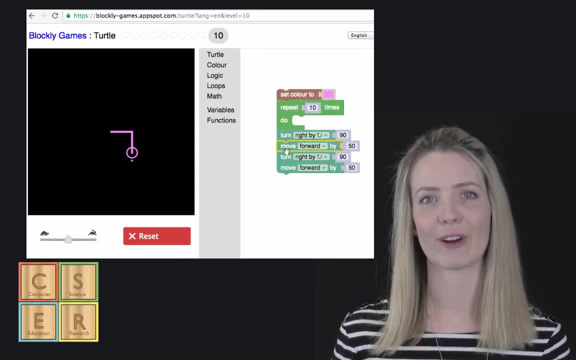 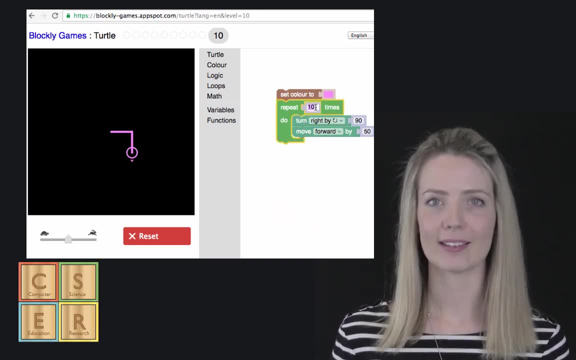 over again. we want to try and think of more efficient ways of writing code. For example, instead of using the blocks write, write up, write, write up. we can recognise this as a recurring pattern. When using visual programming languages, we can use pattern recognition and use techniques. 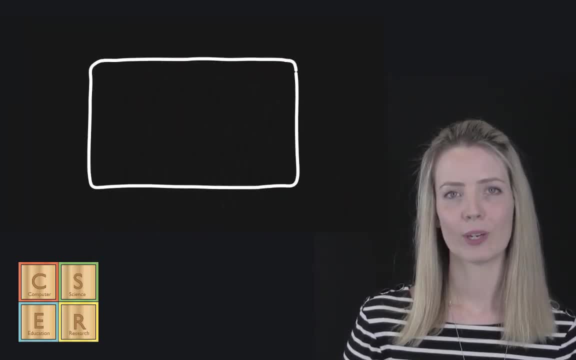 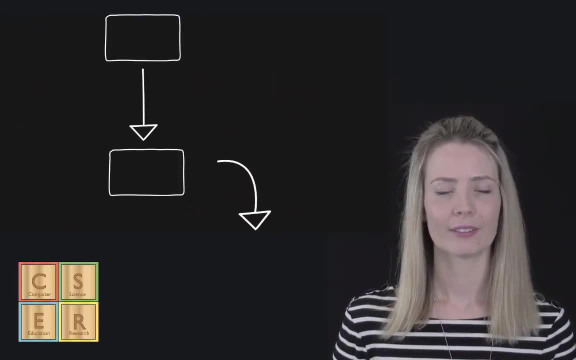 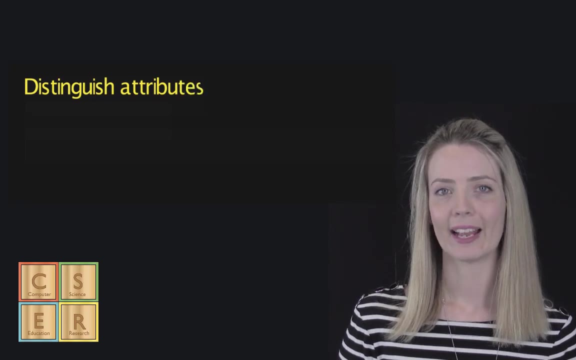 to make the code more efficient. When it comes to designing algorithms, we can examine our designs and consider ways to make them more efficient. There are particular stages of pattern identification. First, we can look at the data or the pattern and distinguish particular attributes such as colour, size and length. We can extract 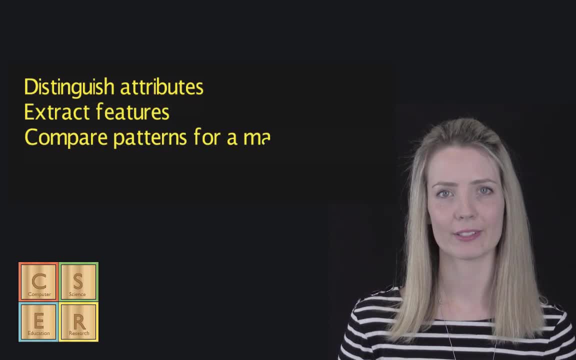 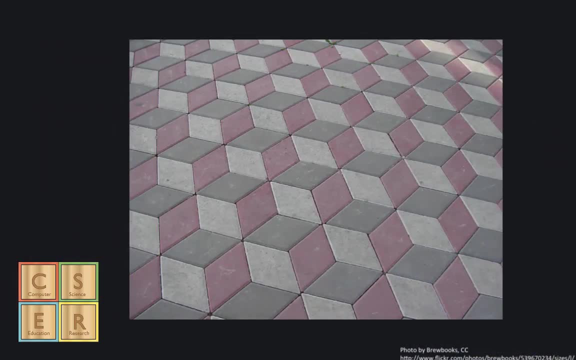 features. And lastly, we can compare patterns to determine a match or a mismatch. Can you identify patterns in this picture? Pause the video and take a moment to explore the tiles. Consider what your strategies are. Think about how you might go about describing this pattern to someone trying to draw an. image based on your instructions. 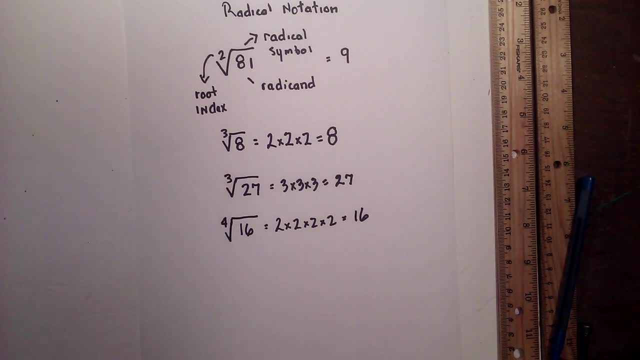 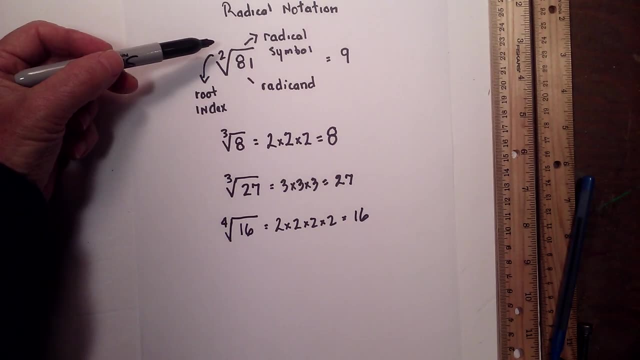 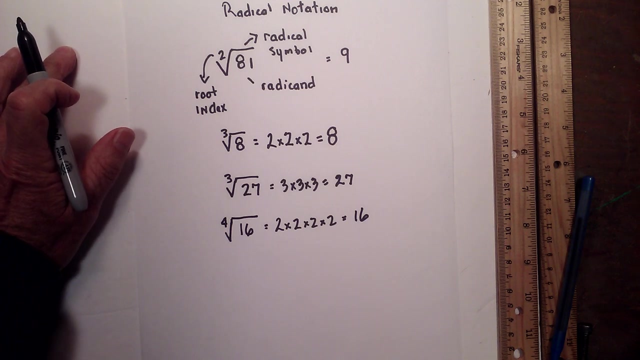 In this video, I would like to talk about radical notation. To begin with, the symbol for radical, which means you are going to take a root of a number. is this symbol right here? Many times, you think of this symbol as a square root only. 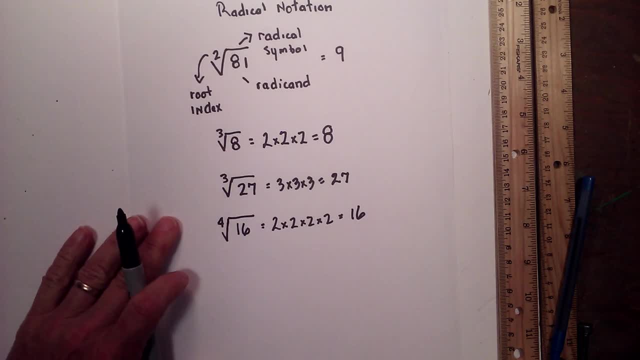 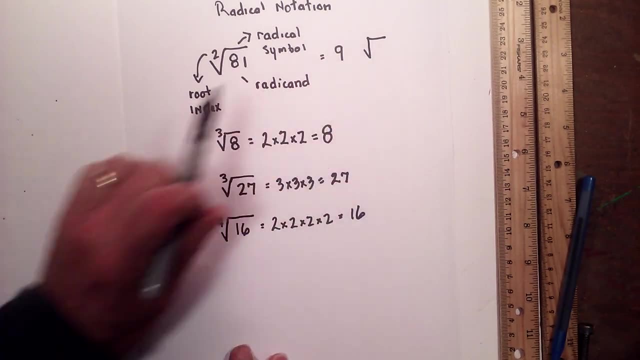 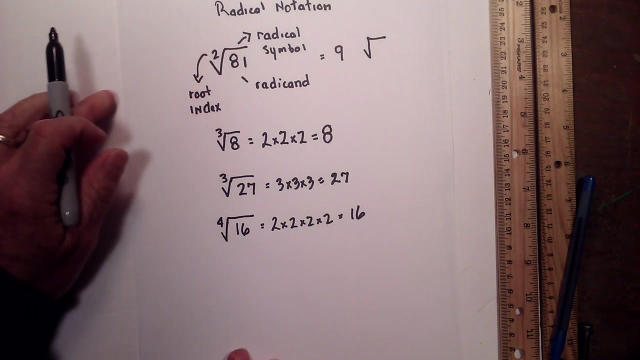 because the root index is 2.. Many times you will see this just written like this and that is a radical symbol and you just assume it is square root. Technically, a 2 would be there. Now what is underneath is called the radicand, and that is the number that you are going.